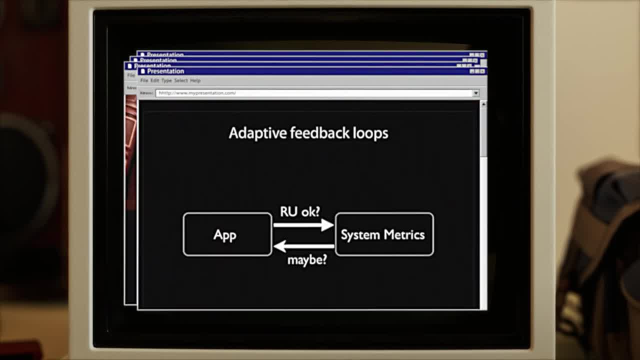 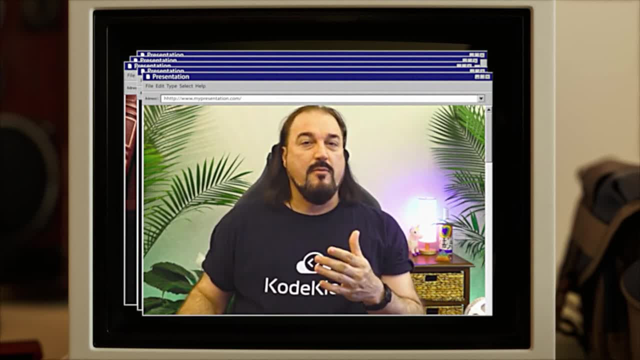 about ideas and perspectives and processes. There weren't really specific technology patterns or usages in the presentation. It wasn't super prescriptive. There was, you know, shared version control was there, as were statements about automation and instant messaging, You know think. 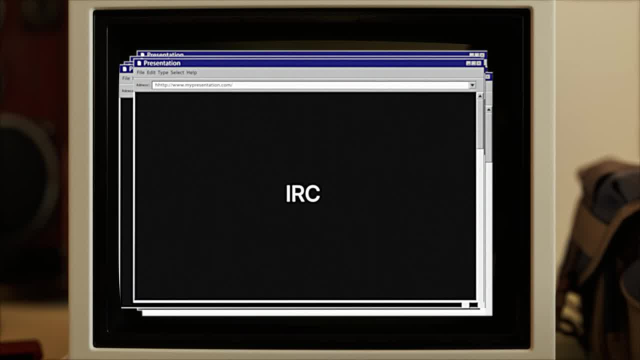 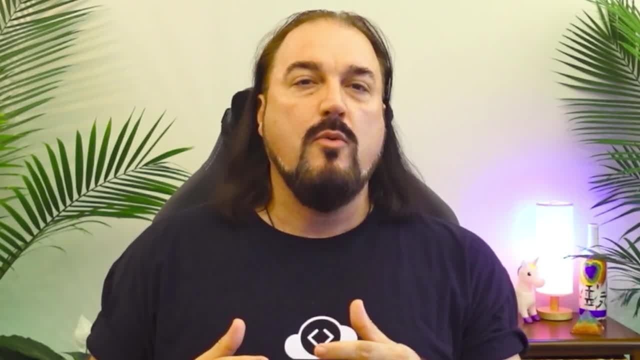 like IRC, for example, which is like old Slack, old Discord in 2022, right, But these were honorable mentions. They weren't really focused on the technologies. They weren't really even that focused on the processes. So what is DevOps if people and processes are the primary message? DevOps is a perspective that eliminates. 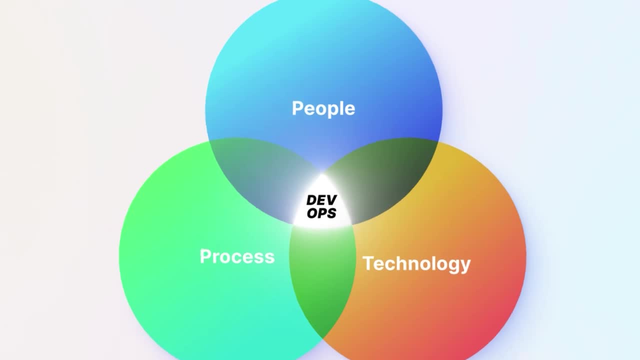 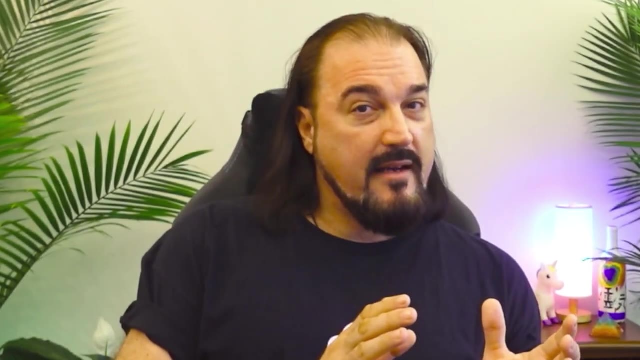 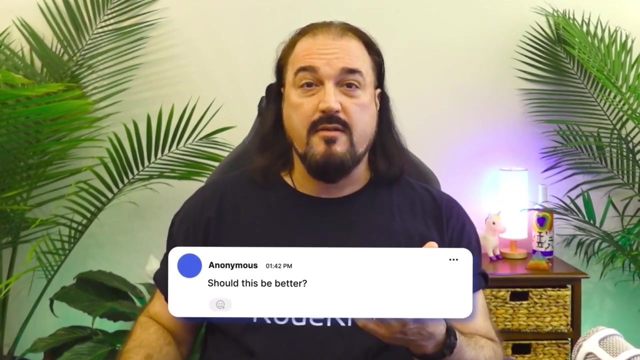 barriers between people, processes and technologies so IT can deliver fast and compliant software to the customer. It's about eliminating the negative to get to the outcome, which is to basically deliver software. Questions like: should this be better, Right? those are common questions. 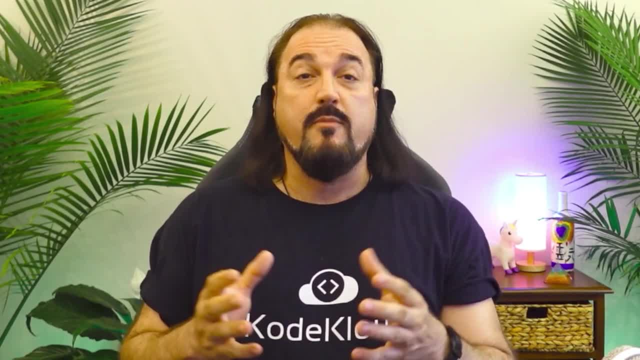 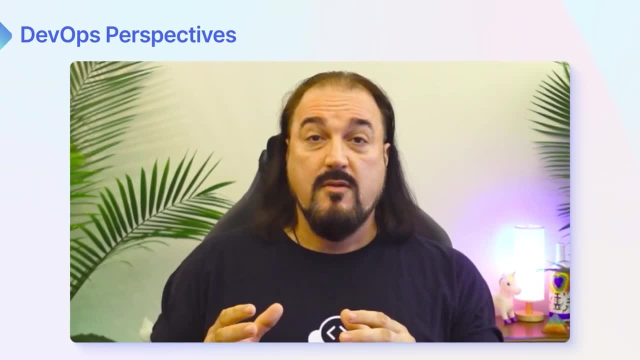 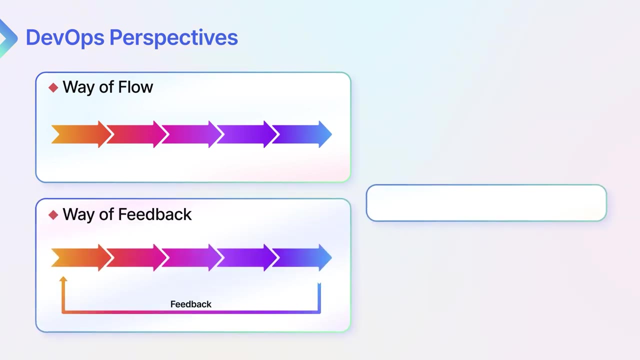 and this is, you know, common. Common for DevOps, for the purpose of evolution and improvement. So DevOps overcomes the barriers by embracing three perspectives. So, when we're looking to remove these barriers, there's the three ways. Namely, there's the way of flow, the way of feedback and the way of continual. 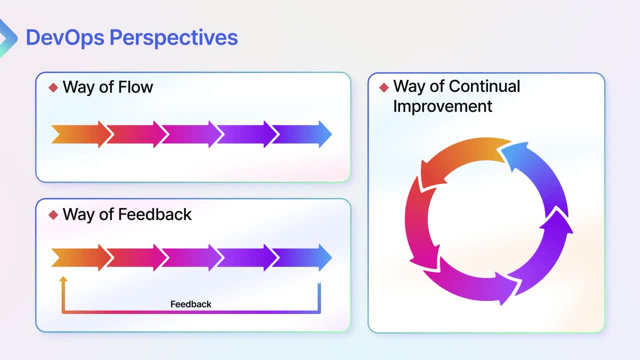 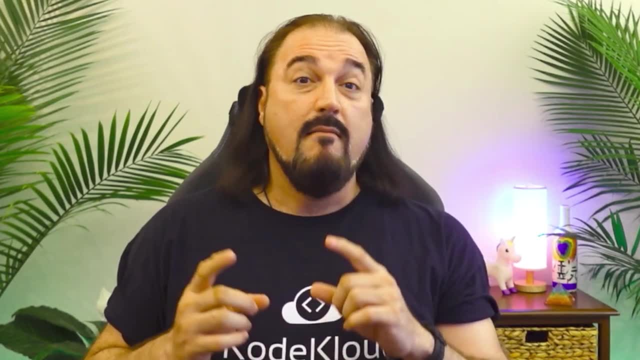 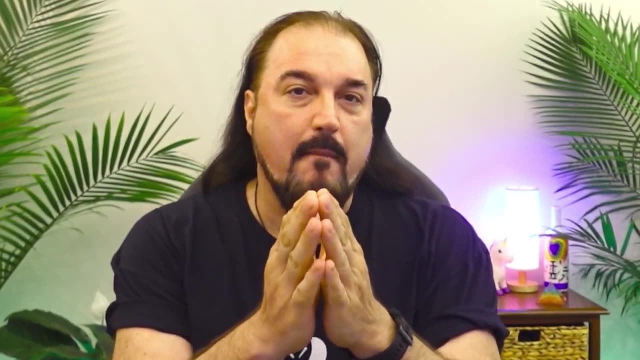 improvement. Now you're going to see a lot more of these concepts in later chapters, but before we get into the patterns and concepts that comprise the DevOps perspective, let's talk a little bit about what DevOps is not. It's hard to define a thing by what it is not, because then that requires us to define all the other things in the 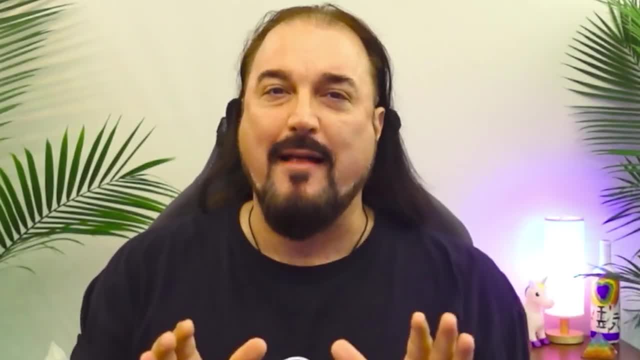 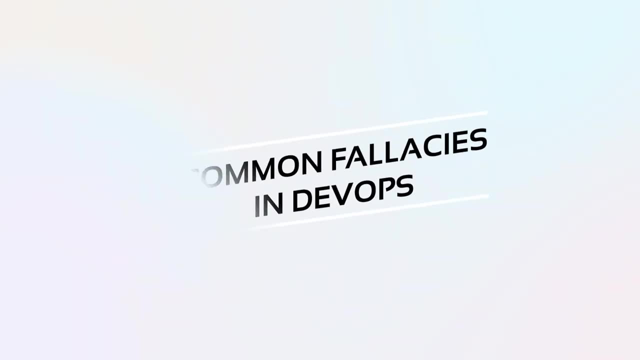 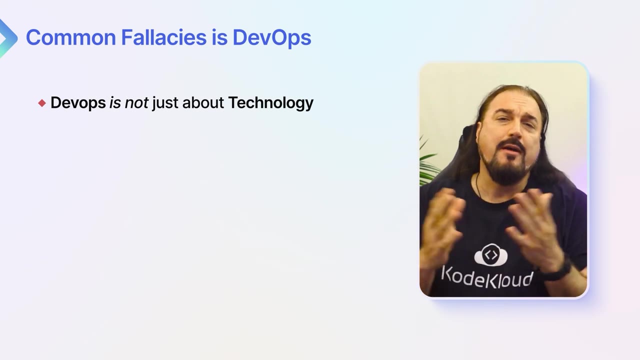 universe other than the thing. But here are some common fallacies about DevOps that should be explored before we dive into those foundations. First, DevOps is not just about technology. Technology comes at the end of a DevOps mindset, not at the beginning. And what good is the best technology in the world if you don't have the right processes and people to? 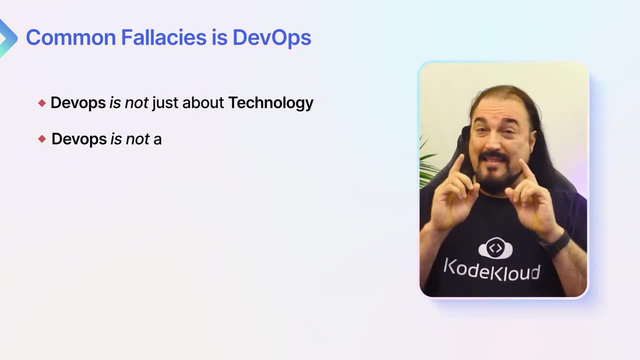 support it, implement it, etc. Second, DevOps is not a job title, So creating collusion among people doesn't happen just because you are titled a DevOps engineer, By the way. nor does having a container orchestrator solve all of your interaction, trust or observability problems. So not a title. 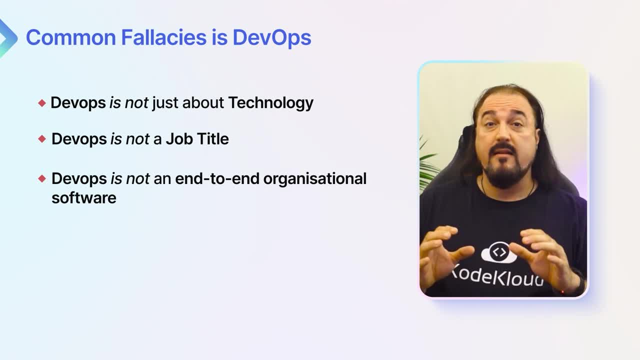 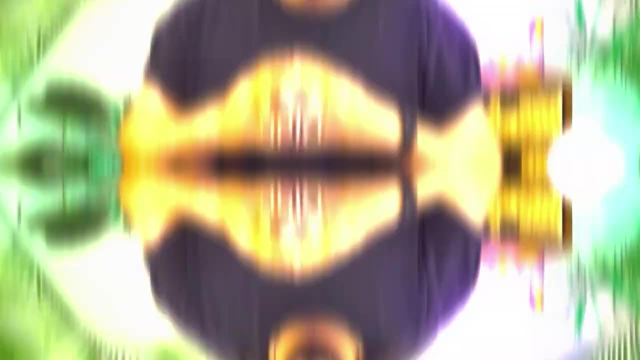 Lastly, DevOps is not a complete end to end kind of organizational software development framework. It has all the components, but it's not a framework in and of itself that you can build on. However, it's easy to understand what DevOps is and it's also easy to know what DevOps is. 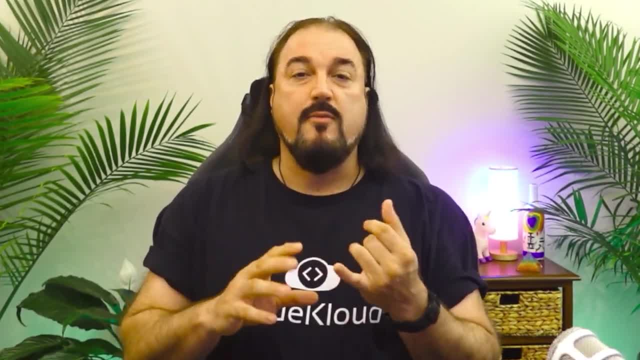 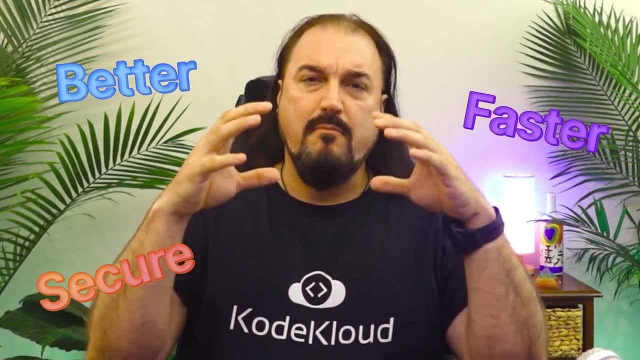 In other words, if an organization is one of the largest and most advanced in the world, it needs to be able to shape and run from the actual field of the organization, It needs to be able to participate in a shared business and it needs to be able to collaborate with the other stakeholders. 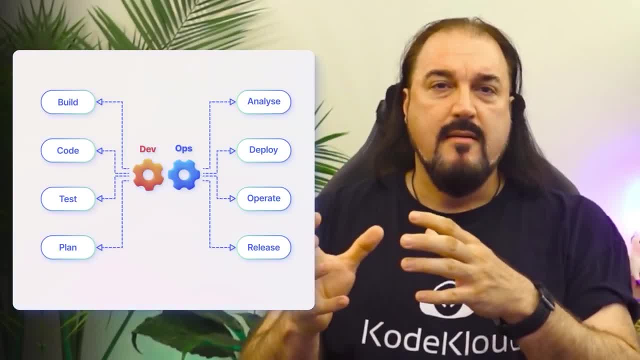 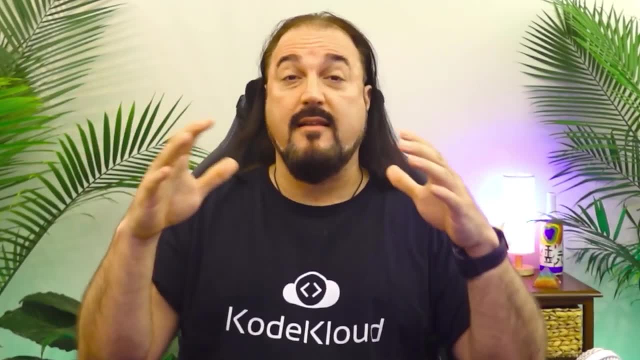 You don't need tools to build the organization that much faster, And the more you understand what DevOps is, the more money you'll be able to make. So this is an interesting area to think about, and one that could potentially be an important insight for some of our audience listeners this week. 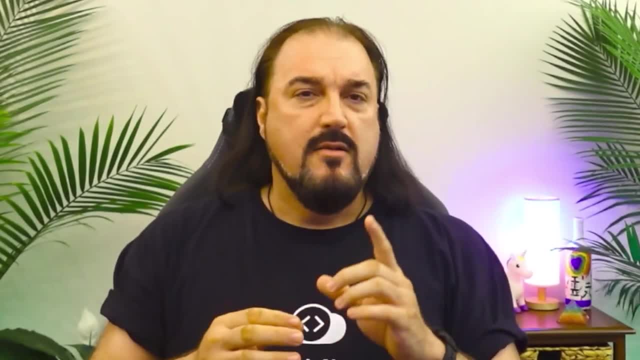 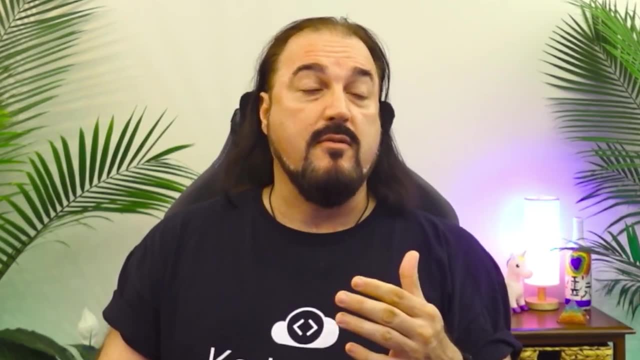 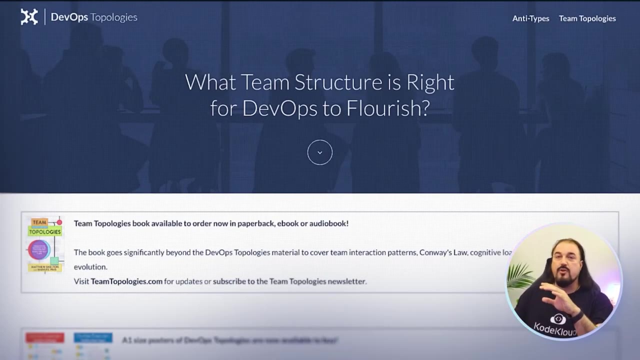 larger framework like agile or scaled agile framework, so let's add a trusted source about devops, teams and organizations. now that we've talked about three common fallacies related to devops, we're going to visit a website called devopstopologiescom, and this website shows: 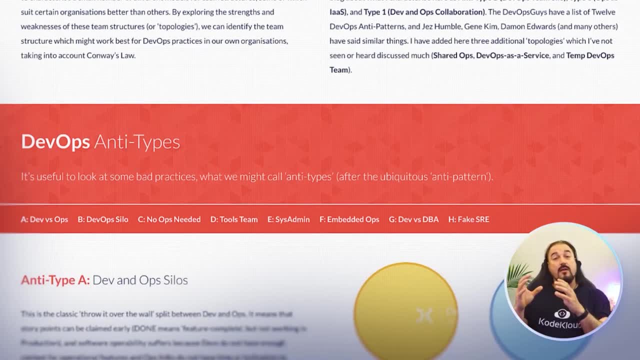 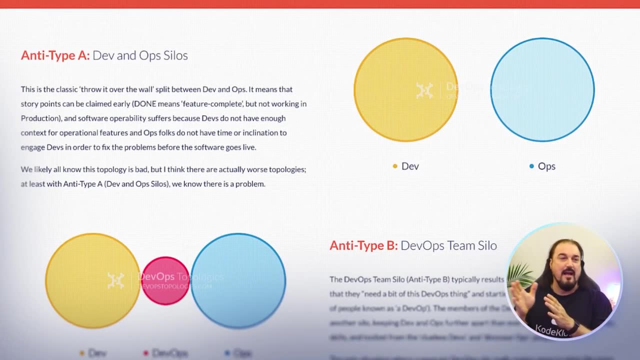 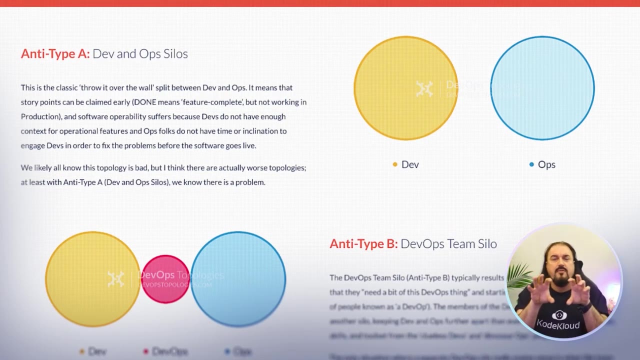 some common anti-patterns that you find in how organizations kind of set up their teams, and so the first anti-type, as you can see here, is the dev and ops silo and you've got dev and operations, developers, operations on separate teams. there's no real close collusion or connection with them. 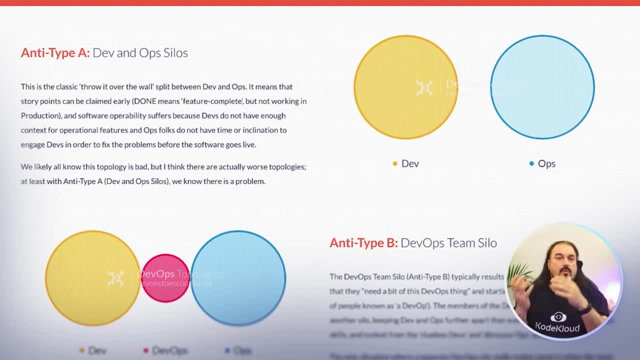 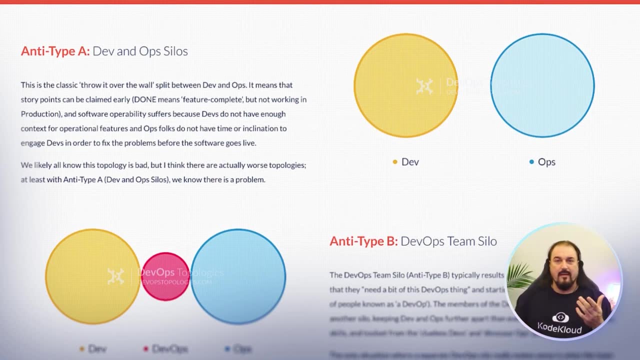 and so you know, developers are just kind of throwing things over the wall at operations. operations is struggling to understand and run them in production and there's no kind of connection or feedback loops there. so that's the first kind of anti-type. the second anti-type is: 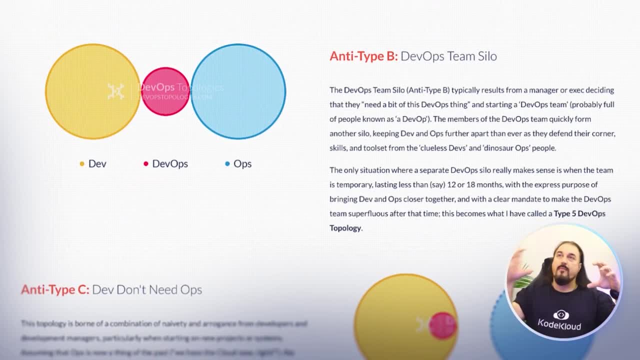 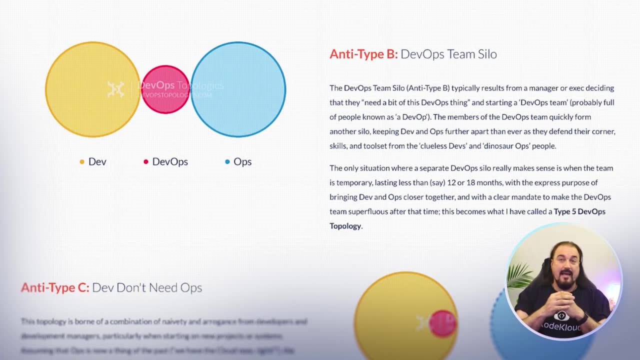 where you organize your teams, where you have developers in a team, you have operations in a team and then you have a devops team and that team's job is to somehow kind of put all that together and that team quickly gets stressed. trying to understand the conflicting, and plus the third, 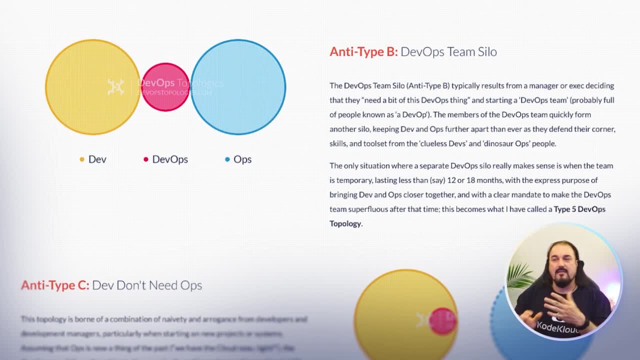 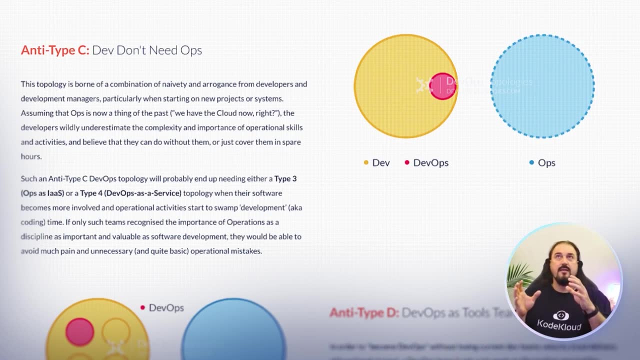 party, and so the whole thing just becomes incredibly complicated, and so this is also an anti-pattern for your devops teams. the third is anti-type C, where devs don't need operations, so they basically take devops and they stick it inside a developer organization. the problem with 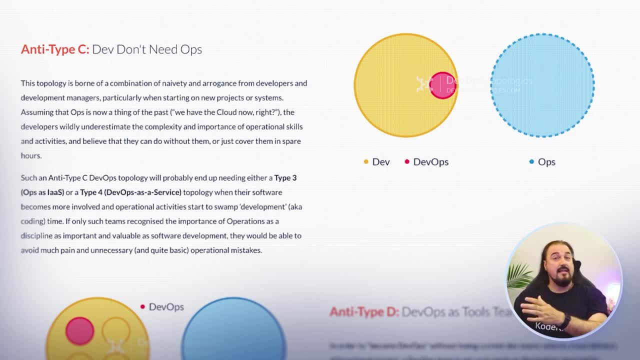 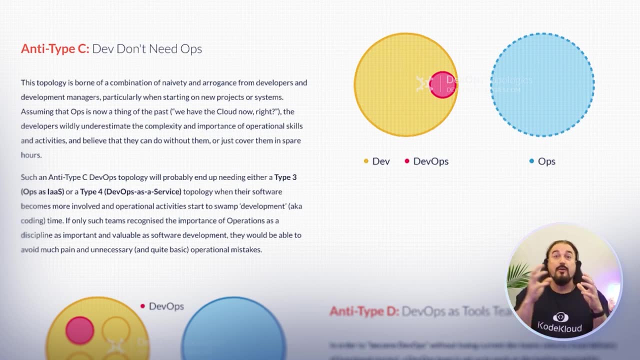 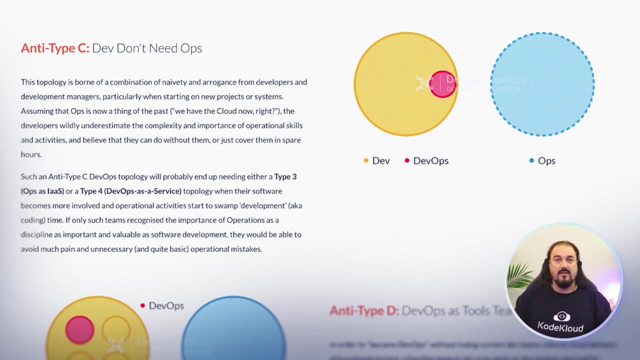 that is that, no matter how smart someone is, is is. operations has very different concerns than development does, and so, while you can embrace that to a certain degree, without actually including operations, you're not going to attend to operational challenges and you've still got this silo, this split in the organization. 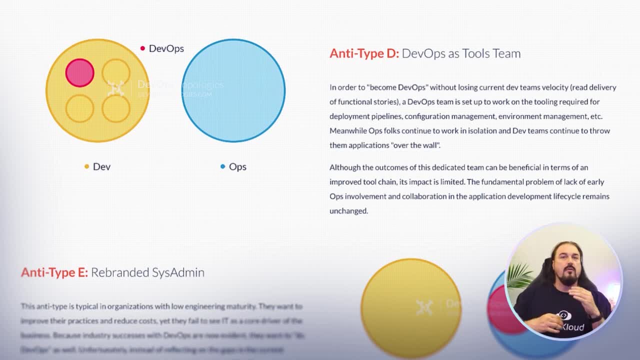 anti-type D devops. as a tools team you know that could work, but you still haven't included operations. operations are still with their own separate concerns and you're not really working with them or colluding with them to capture what their concerns are and I'll go back to to the next question. I hear you have more phangas in your group than before populations right now. I want to chair that. I heard that this isn't asές theеты is likely to be a problem for any of the development teams here at devops. the more I've heard of you views on development teams that you tell me a lot is that. 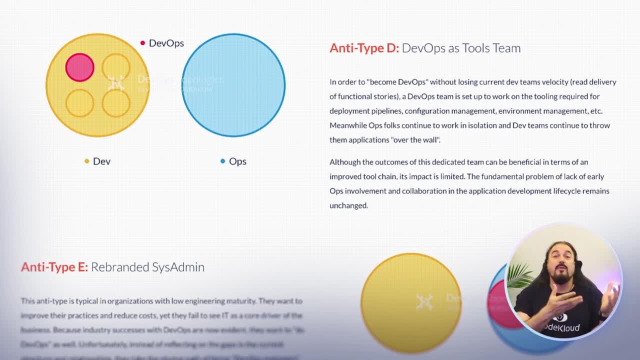 the industry that you asked about, development is highly relatives. Silicon Valley is one of the things their concerns are and allow them, in a way, to help you speed your delivery into production. anti-type e is very similar to the last anti-type that we're going to see, which is basically that. 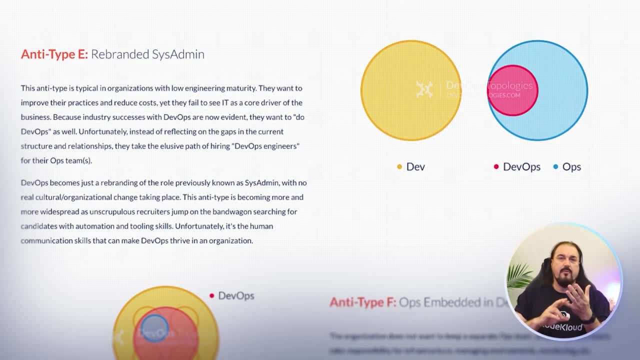 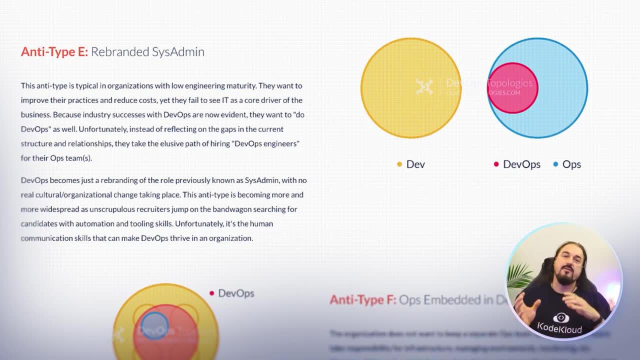 we took a bunch of sysadmins, we didn't teach them about collaboration and automation and collusion and all the stuff that you're about to learn, and we just rebranded them as sysadmins. that obviously doesn't work, because you've got this old sysadmin mindset- kind of i own it, you know. 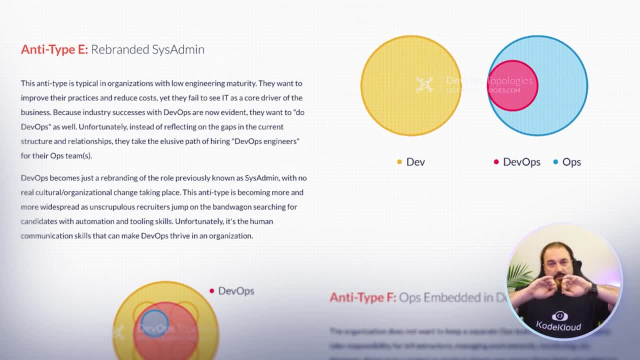 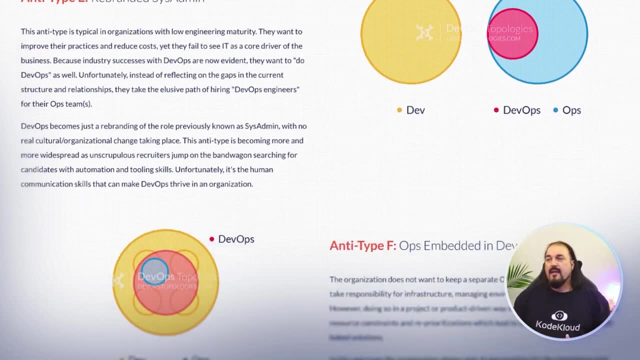 i'm not really involved in the software development process and you've got this kind of wall where you've moved devops into operations but you really haven't created collusion or connection between your teams. anti-type f is our, one of our last few, which basically is where you take. 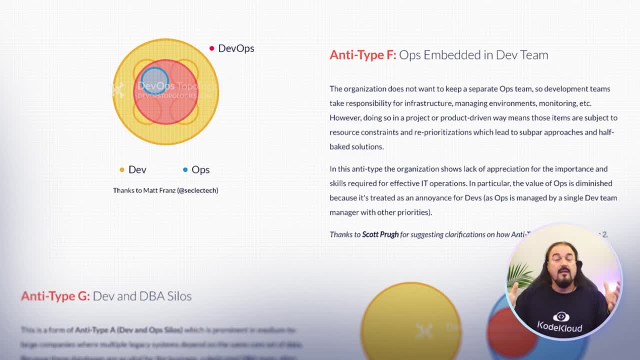 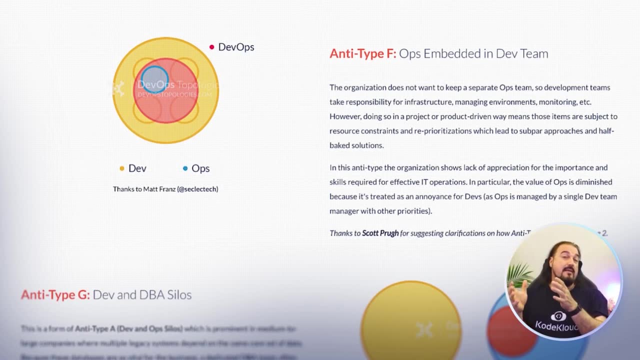 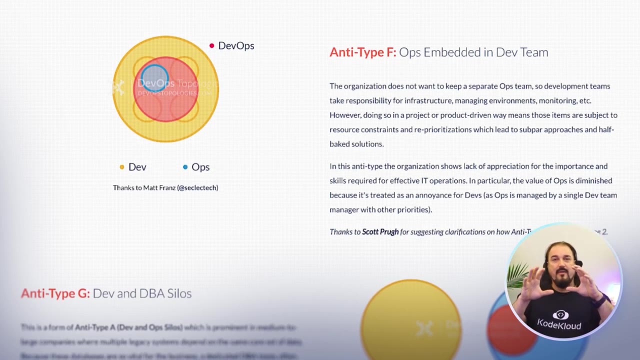 everything and you just embed it inside of a development organization. problem with that is that development organizations are run by development managers, so their concerns are mainly to deliver software, not necessarily to maintain, patch, secure, keep up software. now, could it grow in that way? sure, if both the operations and the devops, concepts and all that 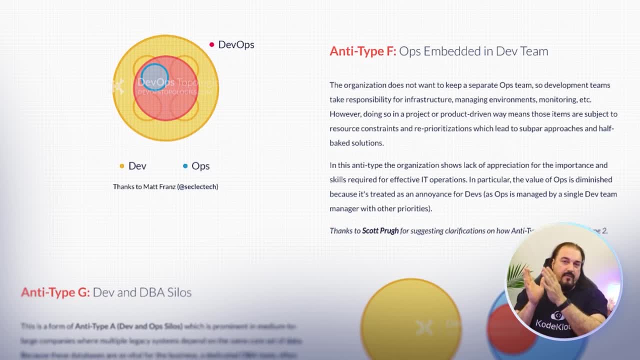 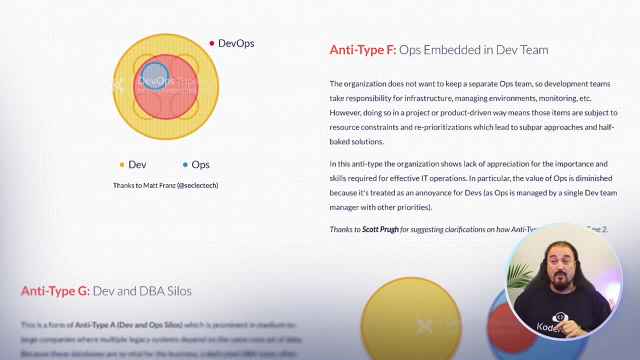 but the entire organization. it could evolve into that, but if developers are in charge, it's not a great thing. if operations is in charge, it's not a great thing. getting the teams to collude together. that's what we're looking for. obviously, that extends over to this next anti-type- anti-type. 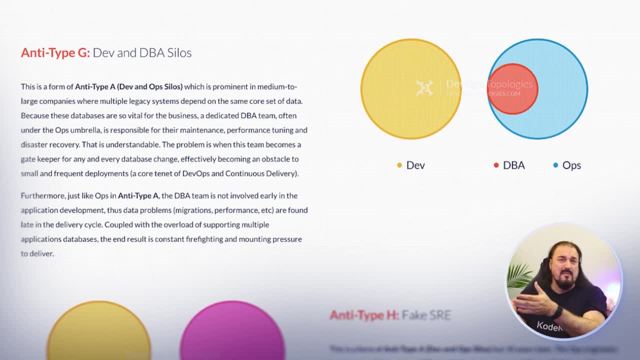 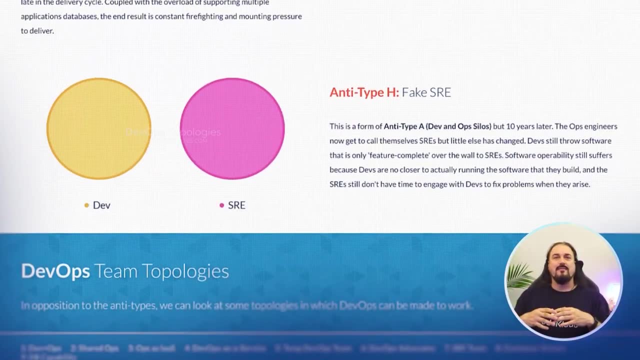 g, where basically you've got, you know, database administrators embedded in operations again. just more silos, more walls, right? this is not helpful, right? and then the last you've got- one that has arisen over the last 10 years- is you've got fake sres, so you've got site reliability. 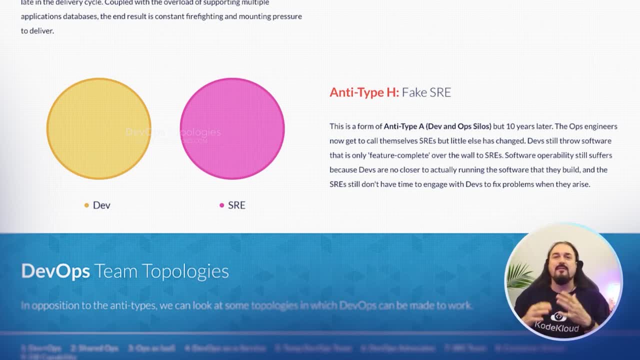 practices and you've got sres that are not trained. they're like old sysadmins who haven't been trained in cyber reliability practices. they haven't done any of the training or any of the work exercises or really just embraced. sre has a discipline and much like non-embracing devops. 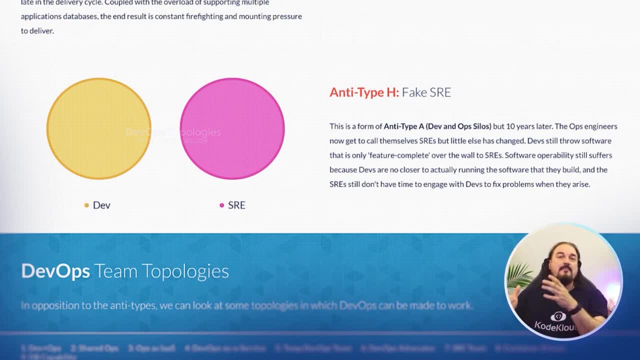 it just doesn't work. you've basically just rebranded your operations team as sres, but you haven't changed them. you haven't changed anything. so keep this in your back pocket. has something to look at when you're thinking about how your organization is structured or if you're an 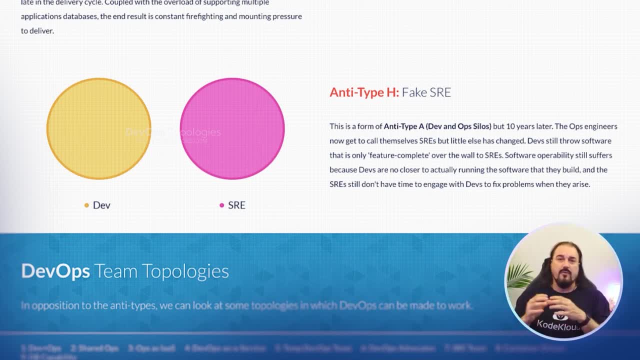 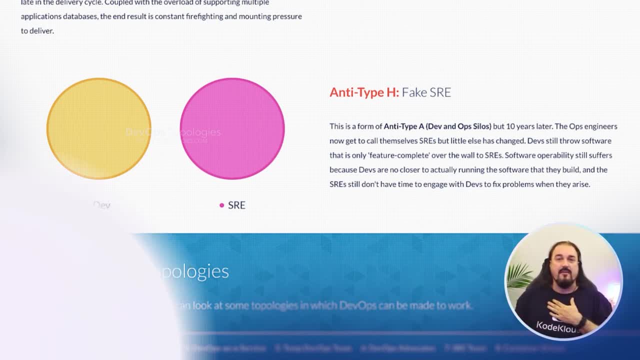 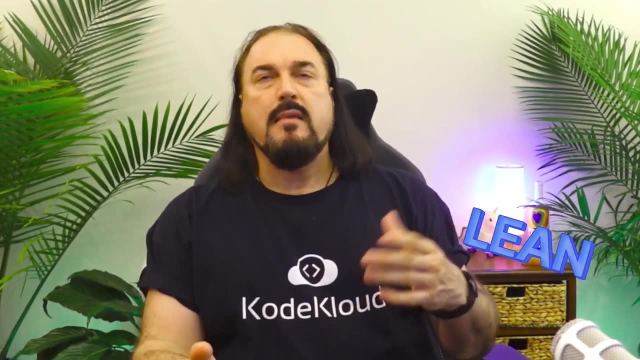 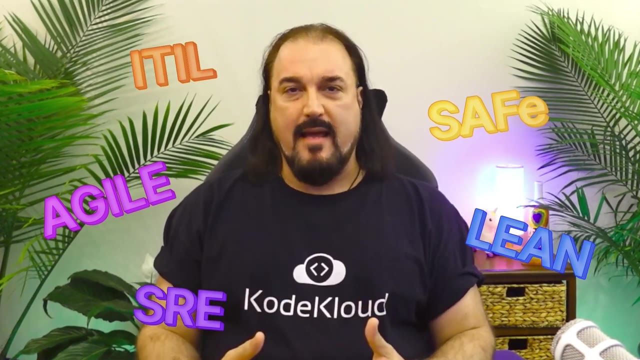 and there's also another page that says what to do. but we wanted to show you some anti-patterns. how does devops relate to frameworks that you might hear about like lean or agile or scaled agile framework or itil sres? others like: how does it relate to that? the simple answer is that, except 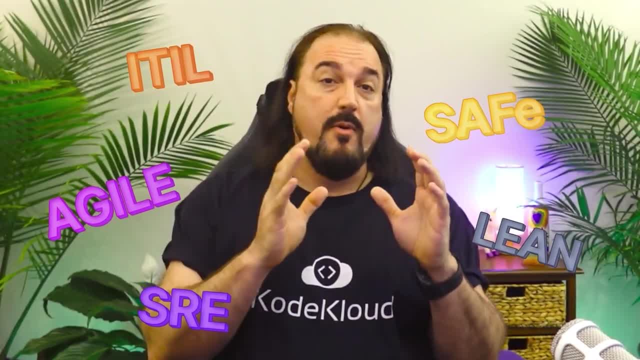 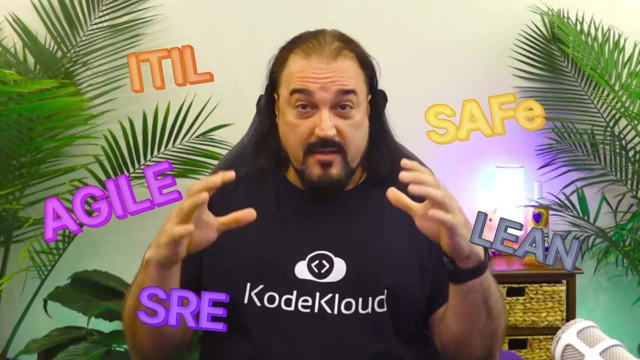 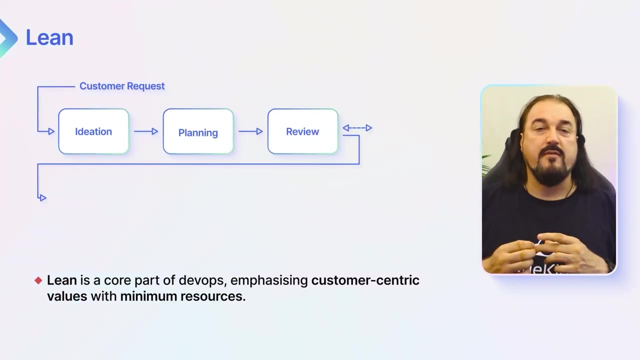 for a lean. almost all other of the frameworks either touch on part of the devops thinking process or some, like the agile flavors, embrace and encompass devops thinking and processes completely, like they pull them into the core. lean is a core part of devops, emphasizing customer. 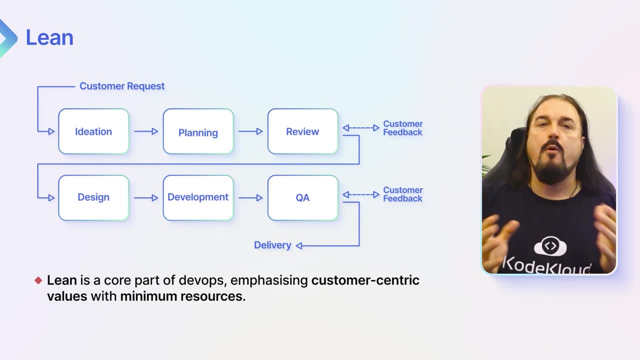 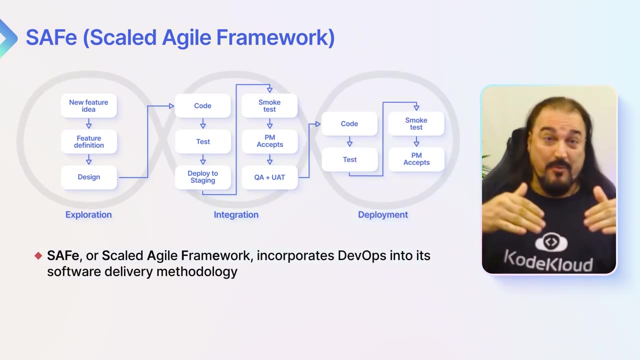 centric value with minimal resources, mainly in small batches, and there's a big emphasis on customer feedback at every iteration of every batch. so, as you can see, lean is kind of in devops safe or scaled. agile framework, for example, incorporates devops into its software delivery methodology. so when it talks about how to provide like for you know. 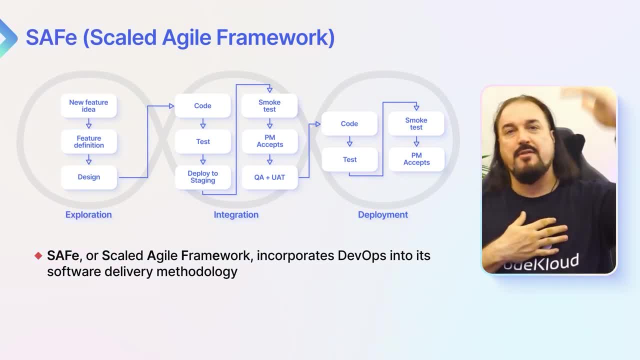 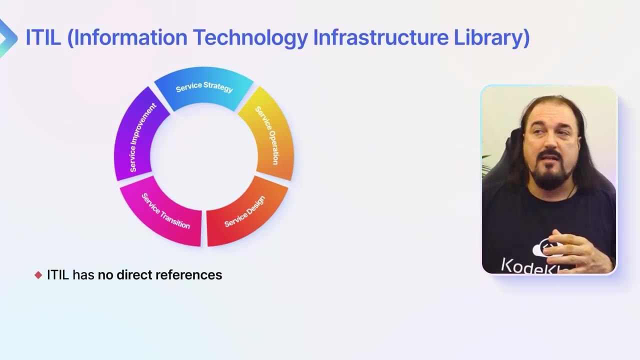 core delivery, where you align strategy to tactics across an entire organization. one of its cores is about value streams, right, and part of that also is, you know, the core around devops. now itil is interesting because itil has no references to devops, yet it defines key areas that are related. 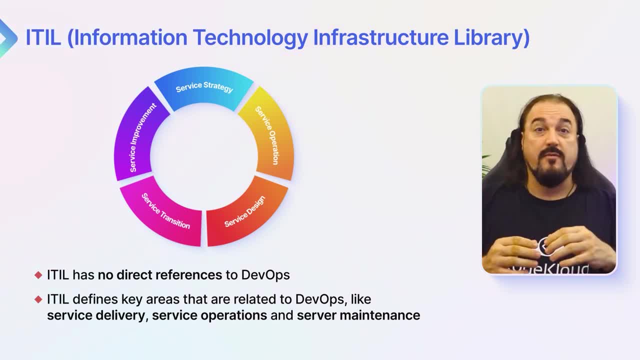 to the devops. like you know, services and things like that, okay, and so, for instance, you now see a delivery and service, operations and maintenance. Those processes have to be put into DevOps to see the flow and do quality improvement that DevOps asks for.